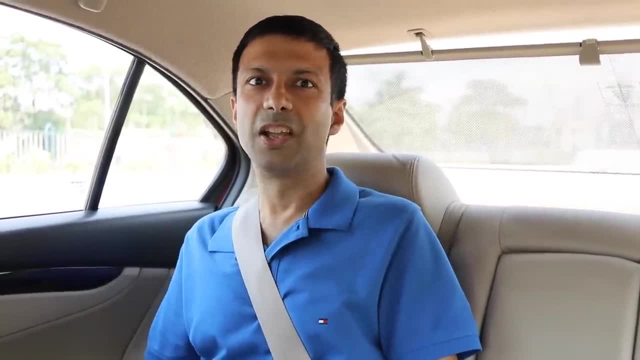 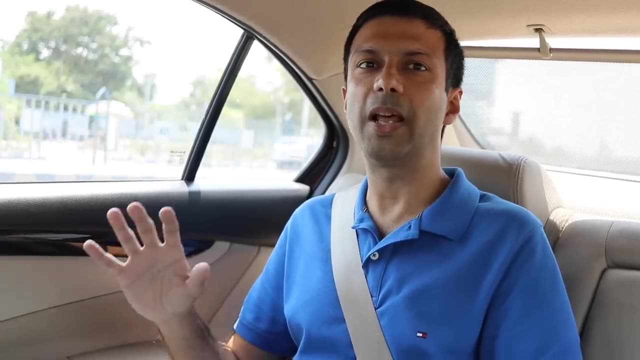 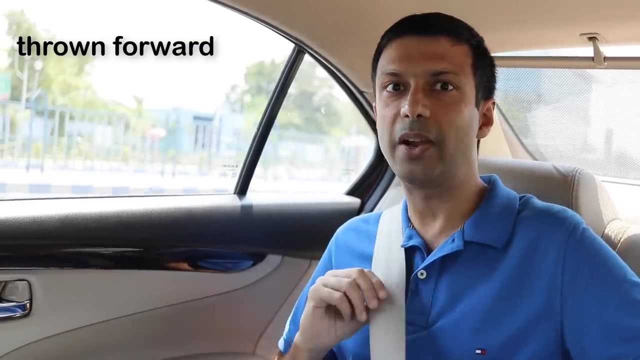 Now let's see how it works. Let's see which law it's based on. Are you ready? Let's go for a drive Now. if the person driving suddenly has to apply the brakes, Did you see what happened? I was thrown forward If I wasn't wearing my seat belt. 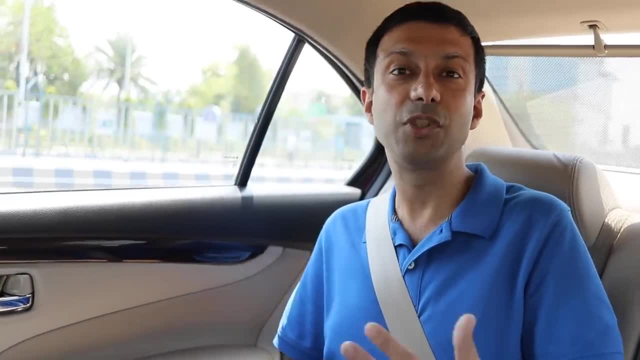 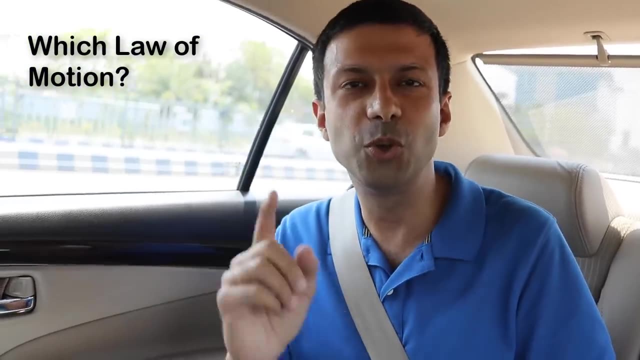 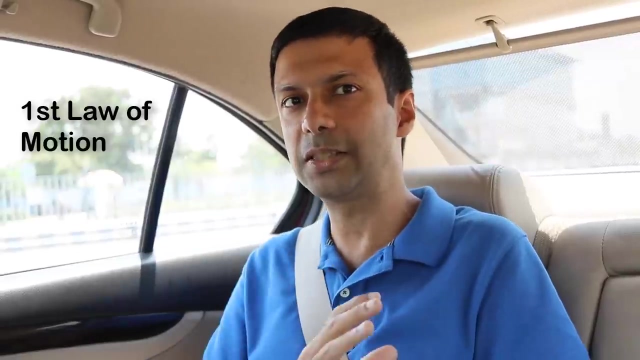 I would have hit the front seat in front of me Or, if I was driving, I would have hit the windscreen. So which law of motion applies to this situation? What do you think? The first law of motion is Newton's first law of motion. This law deals with the inertia of rest and inertia of motion. 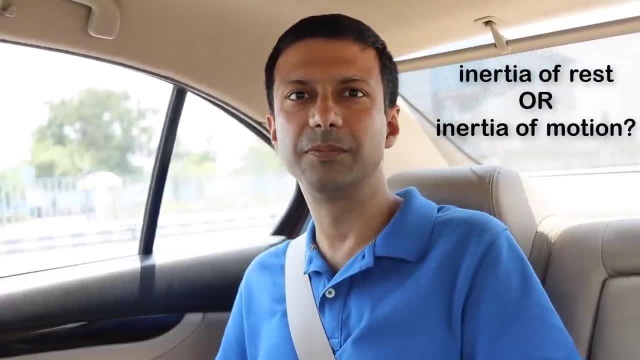 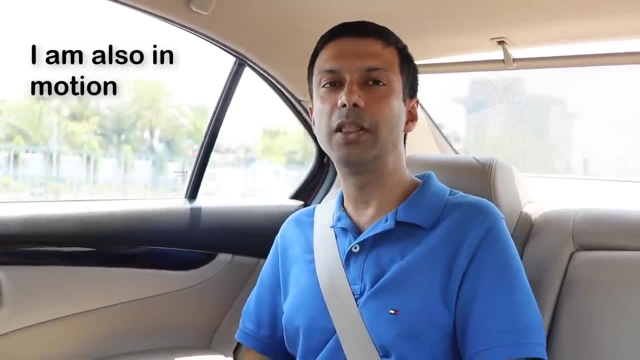 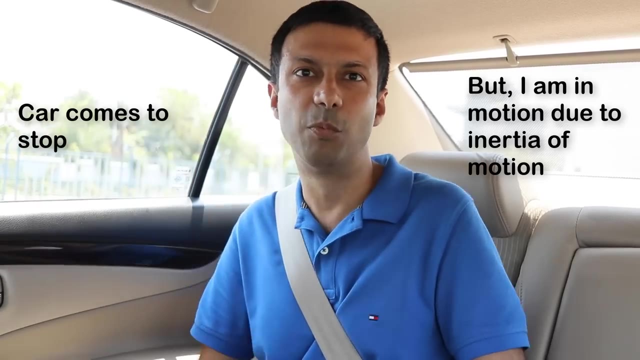 Now let's see which type of inertia applies here When the car is moving. since I'm sitting in the car, I'm also in motion. Now, when the brakes are applied, the car comes to a stop, But I'm in motion due to my inertia of motion. 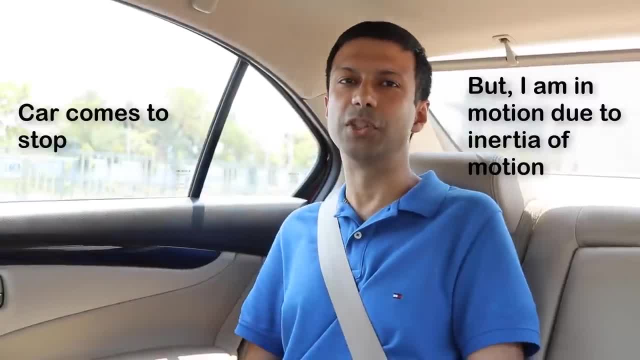 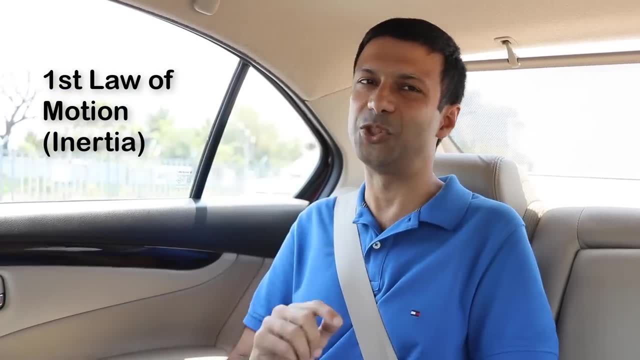 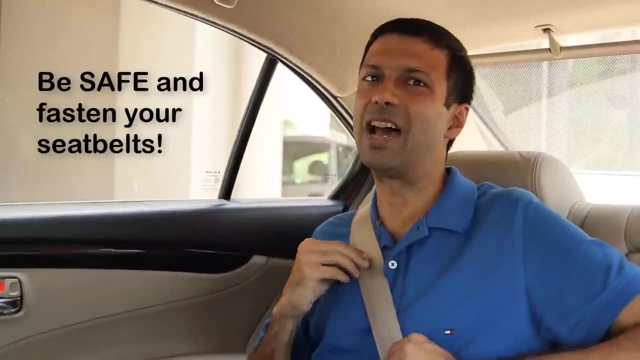 So I get thrown forward due to the inertia of motion. So it's Newton's first law of motion that talks about inertia which applies to this situation. Now I've reached home. So what's the moral of the story? Always be safe and fasten your seat belts. 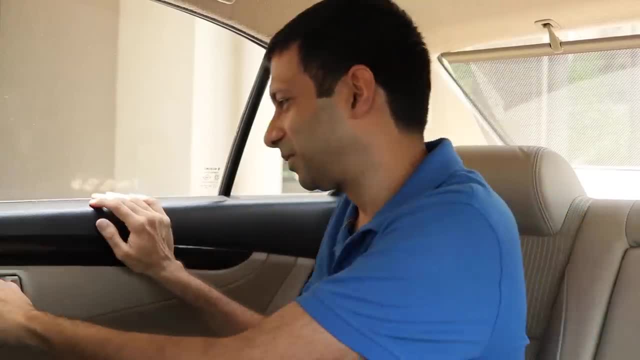 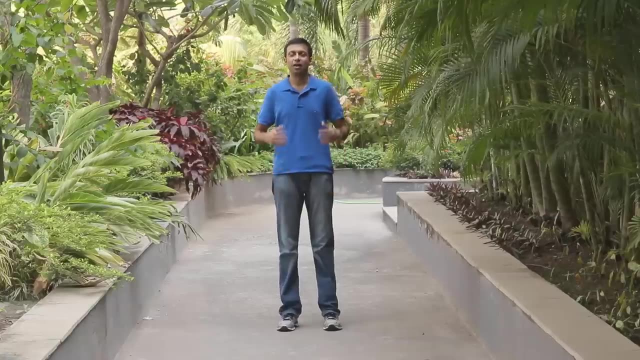 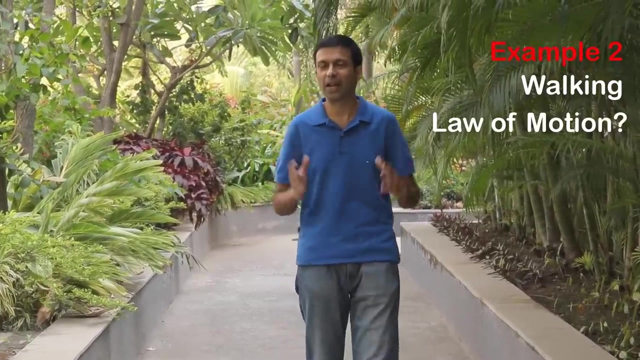 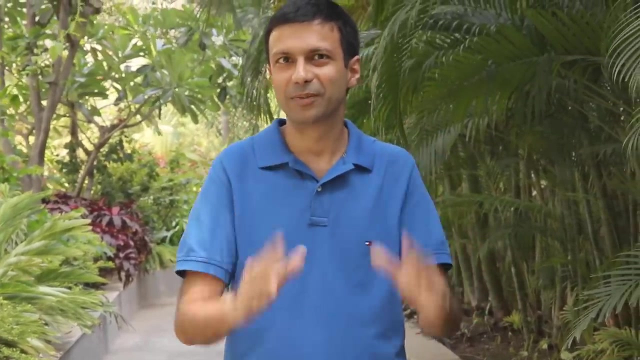 I'm going to get off now and go for a walk. Now let's look at a simple example such as walking. So, while you're walking, which law of motion applies here? That's right, It's Newton's third law. Now let's take a closer look. 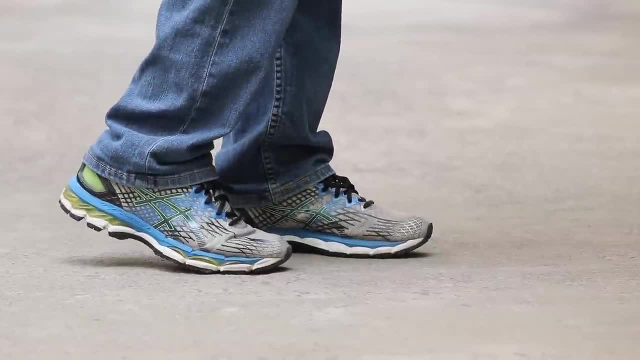 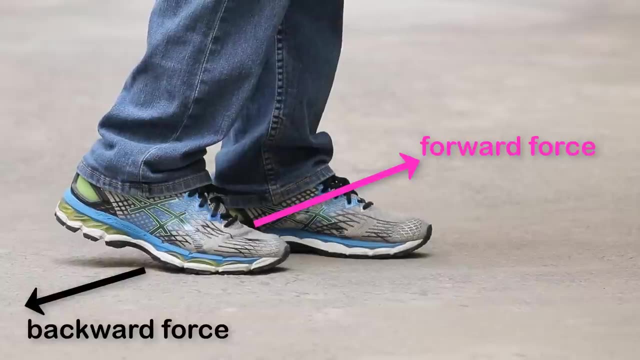 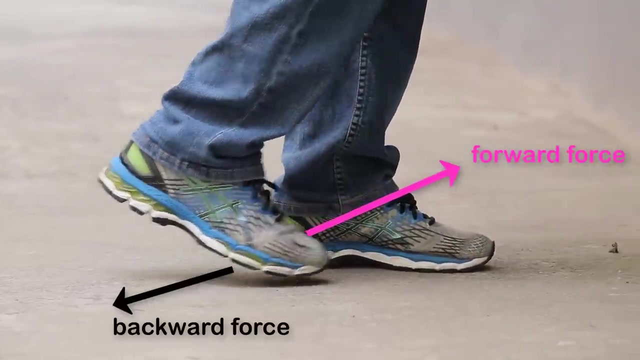 When you're walking, your feet are pushing the ground. Your feet are applying a backward force on the ground. The ground, in turn, applies a forward force on our feet, pushing us forward and making us move. Can you see the action-reaction pair? 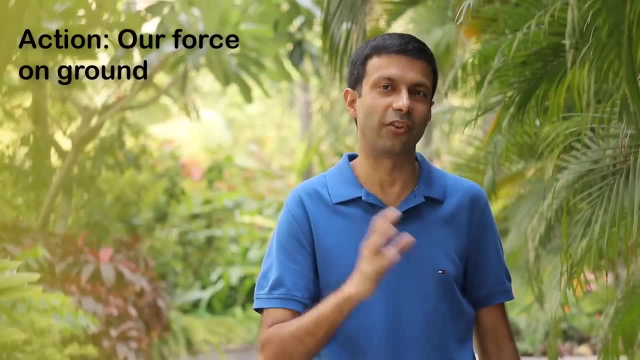 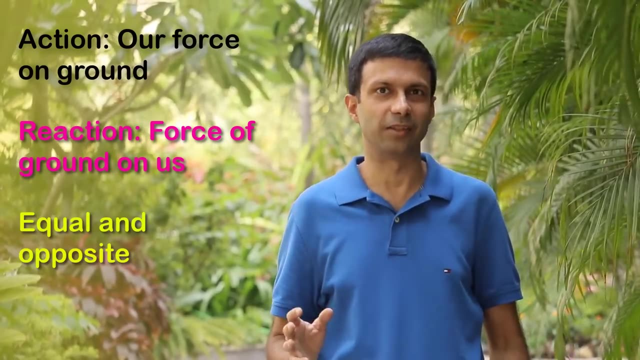 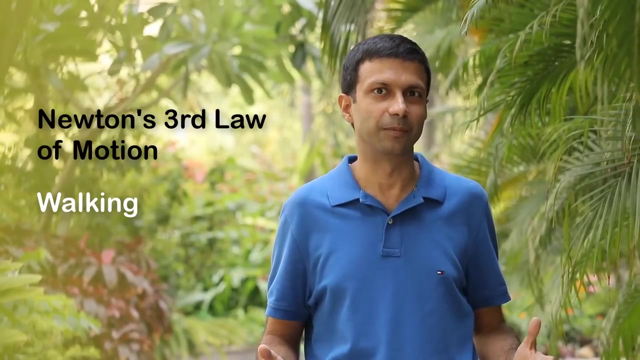 Action is our force on the ground and reaction is the force of the ground on us. The two are equal and opposite. So it's Newton's third law of motion: Every action has an equal and opposite reaction, And this law explains how we walk. 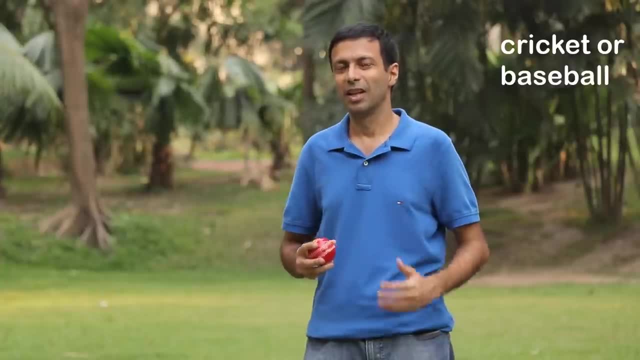 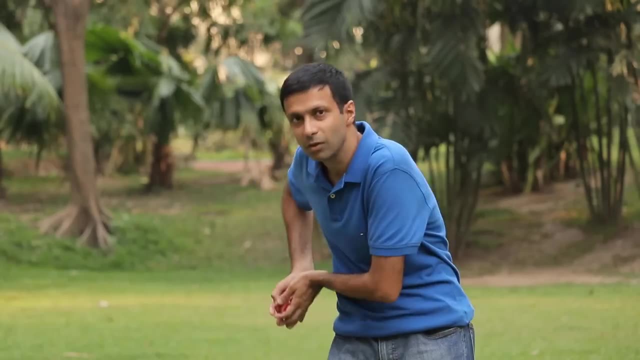 Let's say you're playing a game like cricket or baseball. Here I have a cricket ball with me. The coaches teach you to take the catch like this, With your hands moving down. But if you take the catch like this, Ouch. 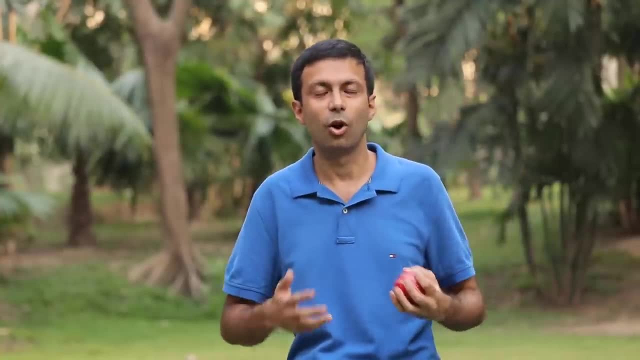 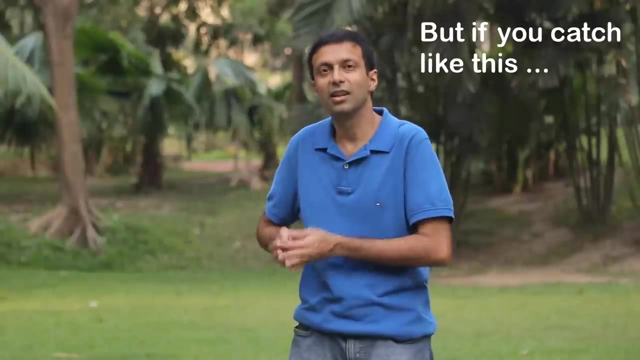 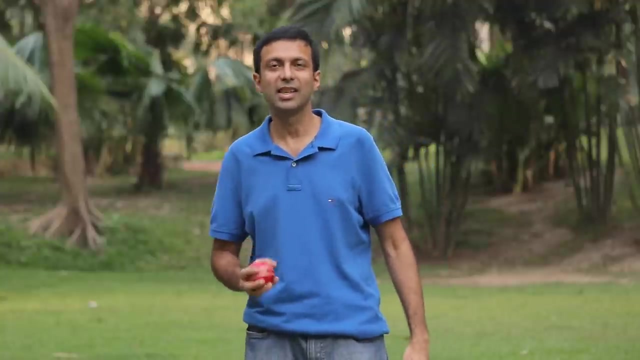 Since the ball is pretty heavy, it can hurt your fingers or it can bounce off your hand, But if you take the catch like this, It doesn't hurt your hand. Why is that? Which law will help us answer this question? To analyze, let's consider some numbers. 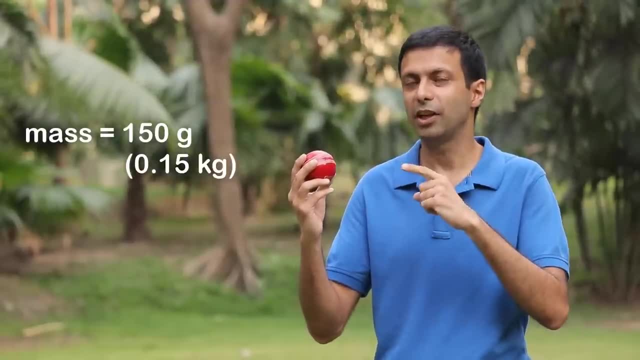 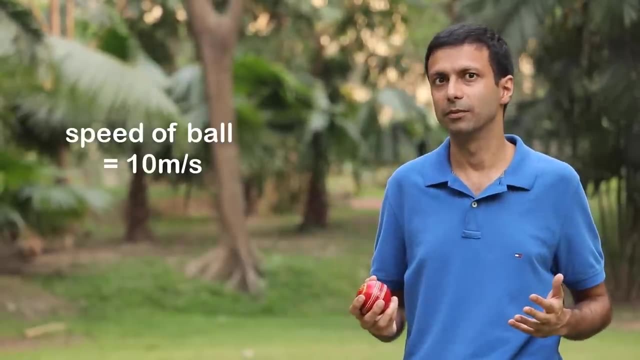 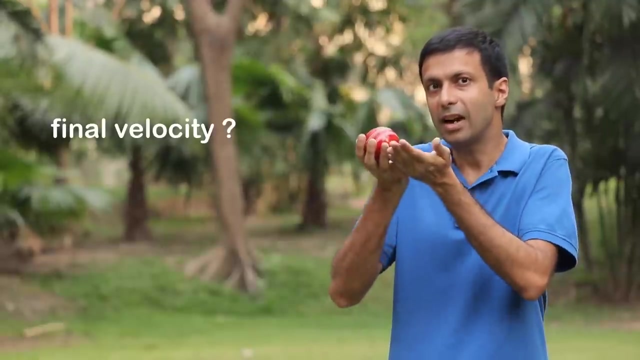 The mass of this cricket ball is 150 grams. Let's say the speed at which it hits my hand before the catch is 10 meters per second. So the initial velocity is 10 meters per second. Now what is the final velocity after the catch? 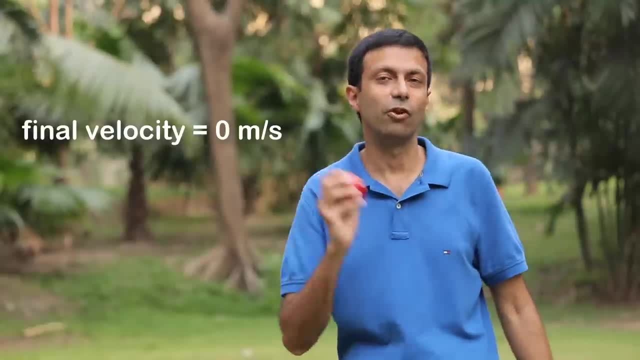 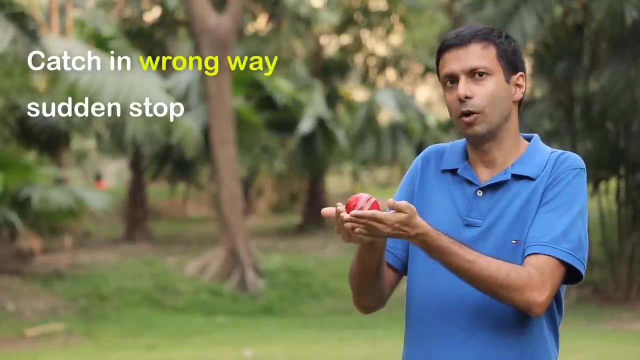 That's right, It's 0 meter per second. Now let's say I didn't take the catch in the correct way, So the ball comes to a sudden stop. In, say, 5 seconds, So the ball comes to a sudden stop. 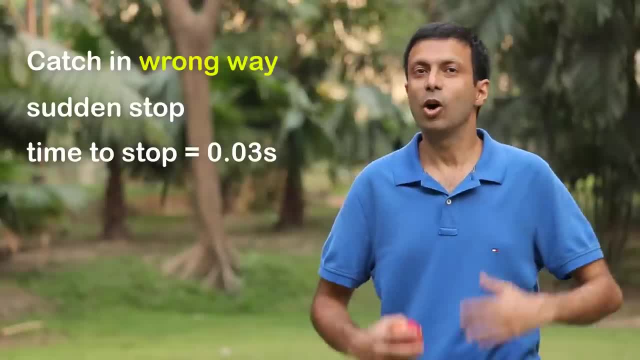 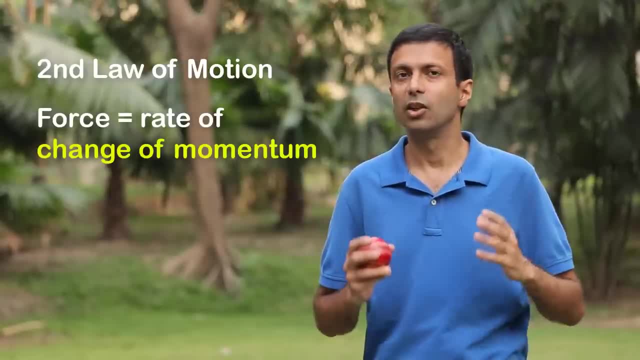 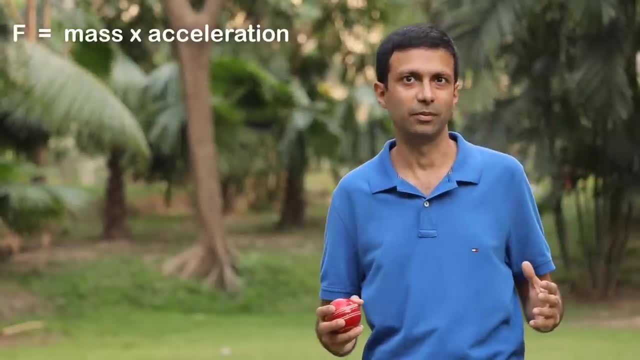 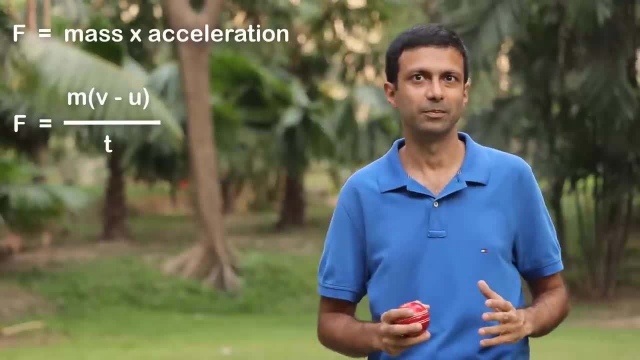 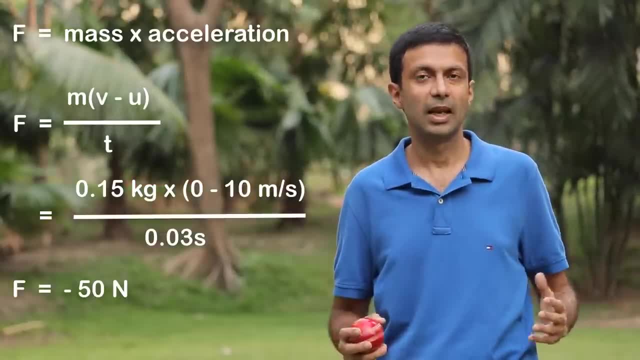 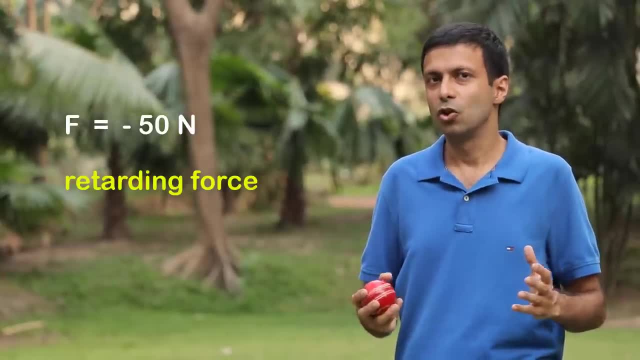 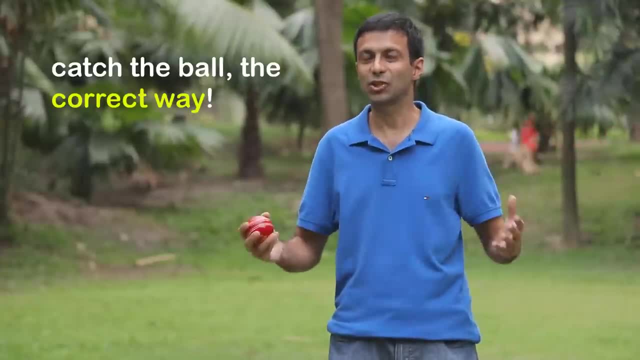 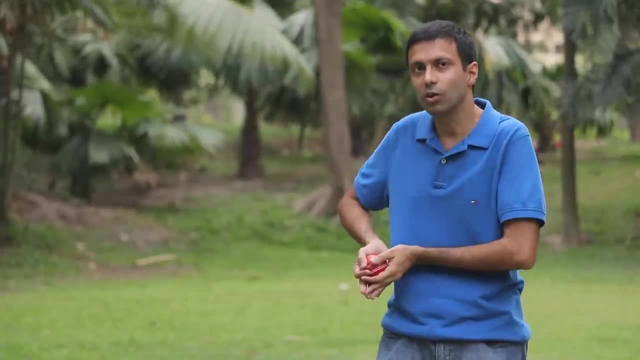 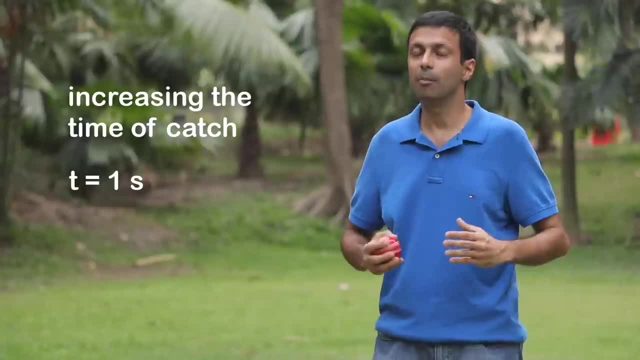 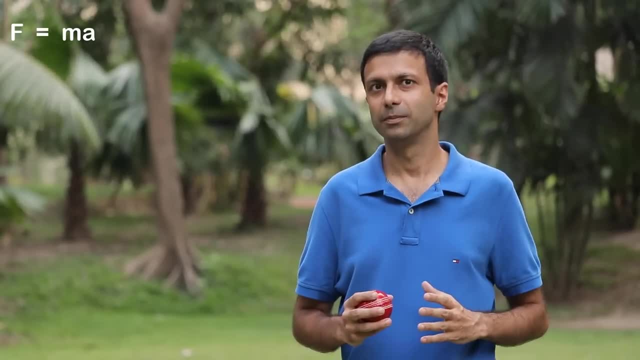 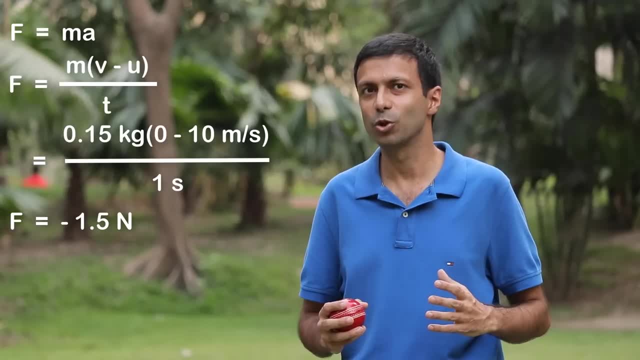 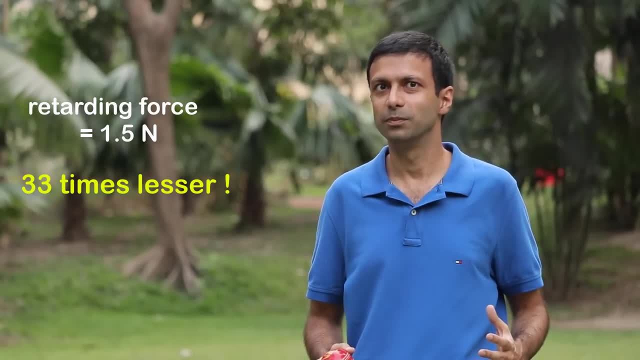 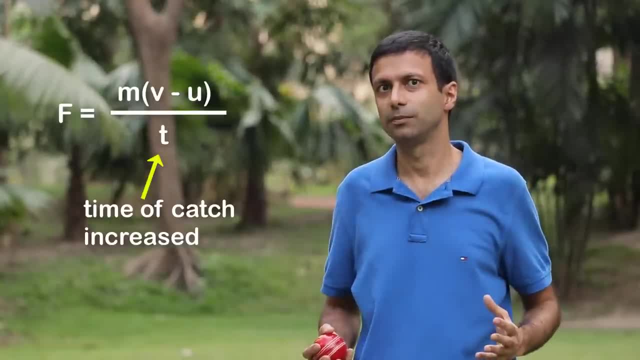 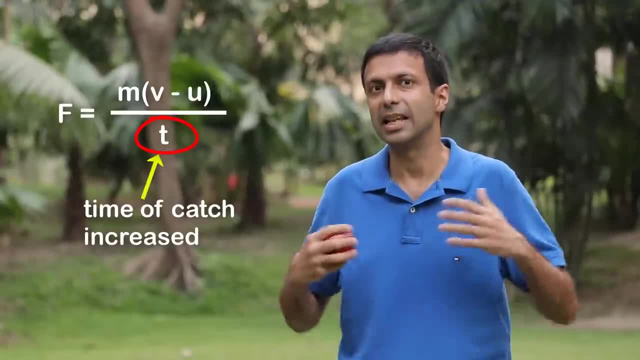 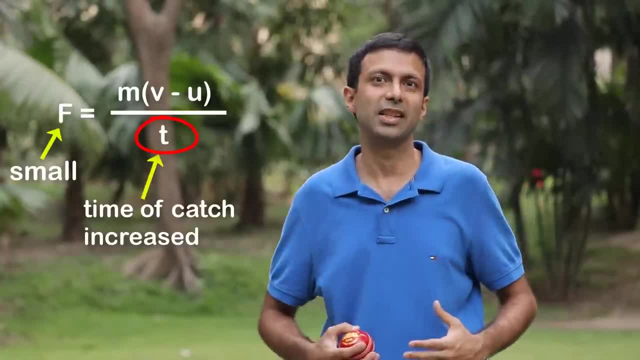 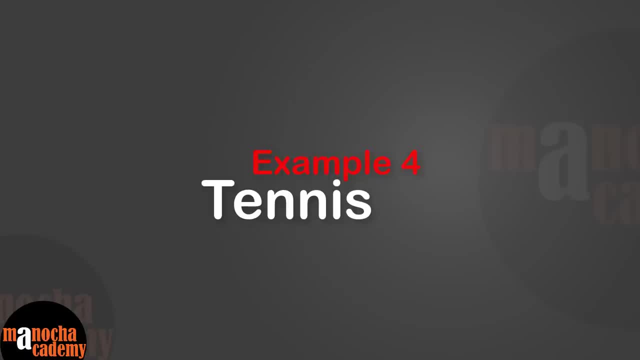 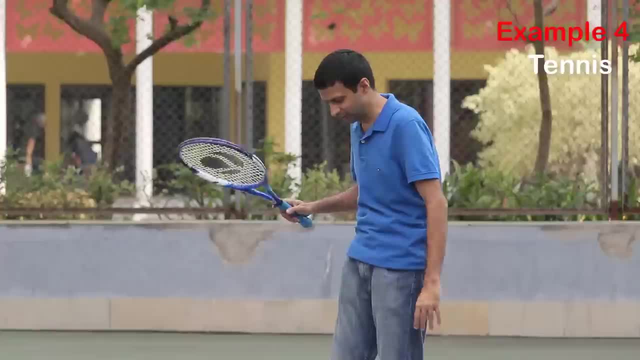 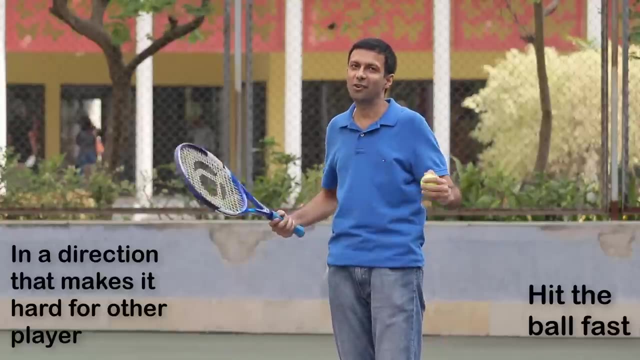 In, say, 5 seconds, So the ball comes to a sudden stop. In, say, 5 seconds, So the ball comes to a sudden stop. While playing tennis, you want to hit the ball fast and in a direction that makes it hard for the other player to get to the ball. 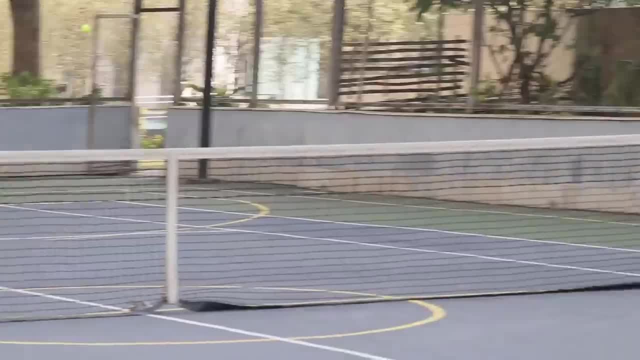 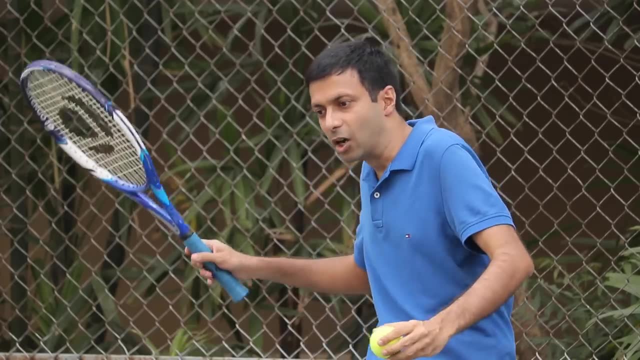 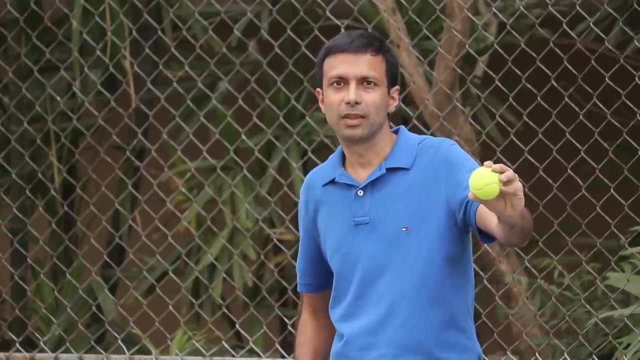 So how do you do that? By hitting it like this. When we want to hit the ball hard and in a direction we want it to go, A greater force causes a greater change of momentum in the ball and makes it go faster. The ball moves in a direction that we hit it in. 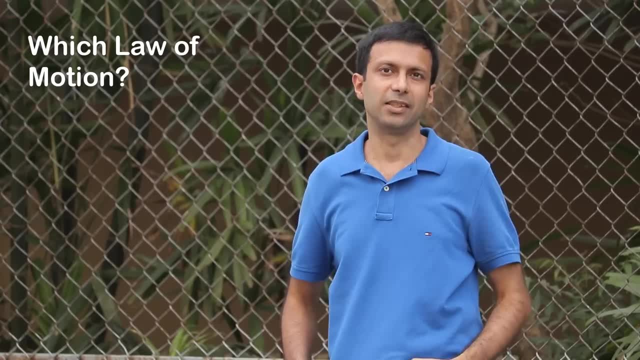 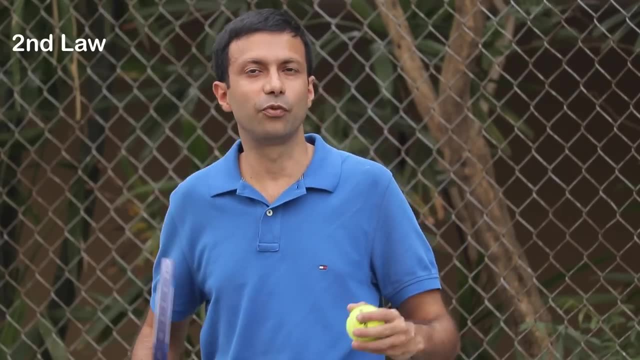 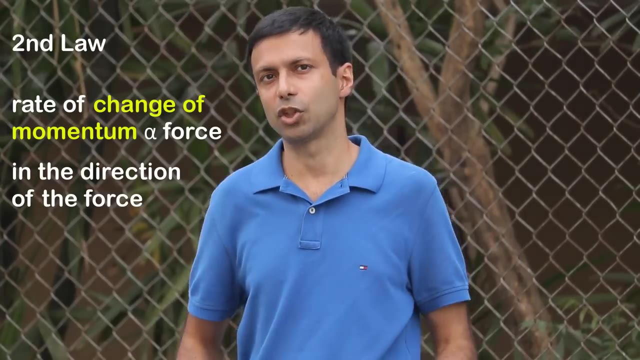 So which law of motion tells us this? That's right. It's Newton's second law of motion, which states that the rate of change of linear momentum is directly proportional to the applied force And it takes place in the direction of the force. 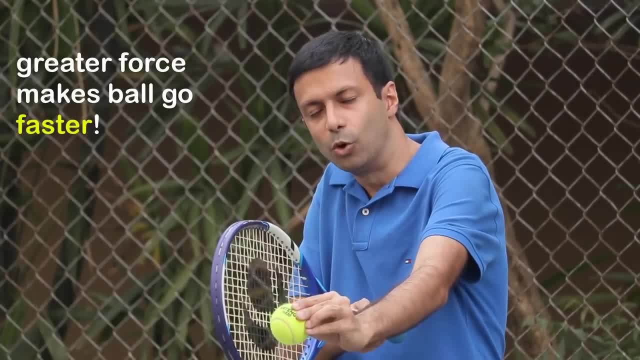 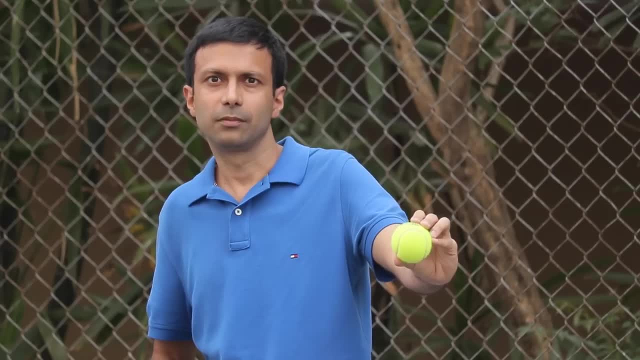 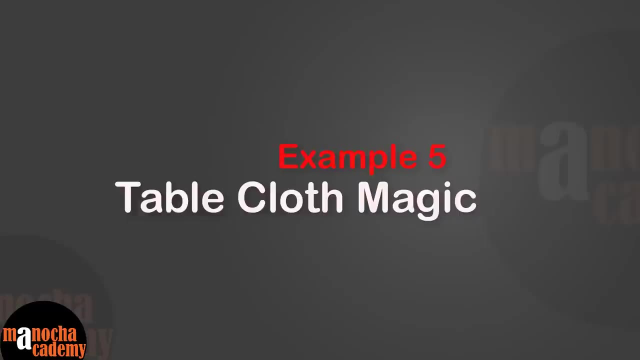 So if you hit the ball with a greater force, the ball will go faster. There will be a greater change of momentum. There will be a greater change of momentum in the ball And the change of momentum takes place in the direction of the force. 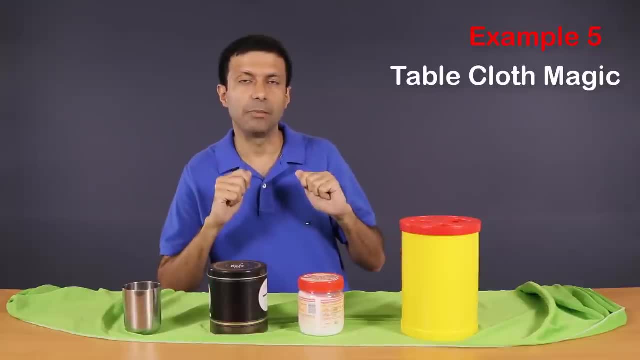 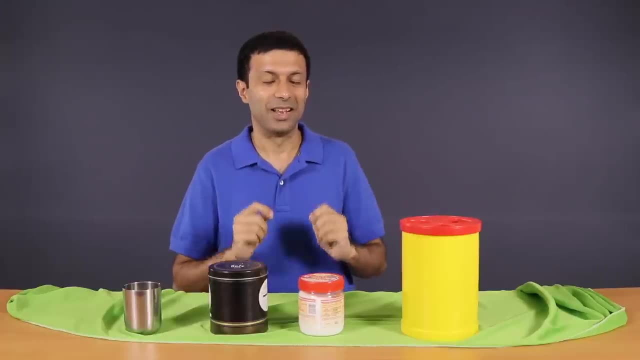 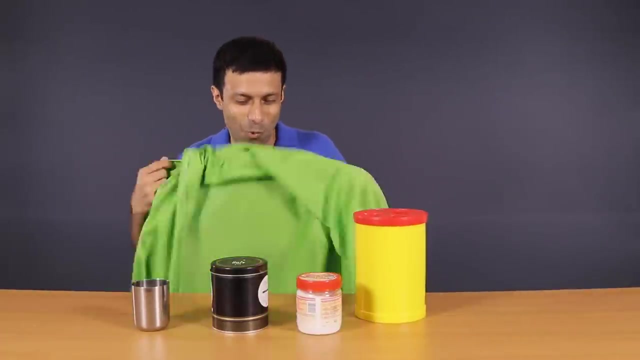 You might have seen this magic trick before, where they pull the tablecloth and the things don't fall. Now, I'm not a magician, so please wish me luck. Let's try. Ready One, two, three, Whoa. I'm happy it worked. 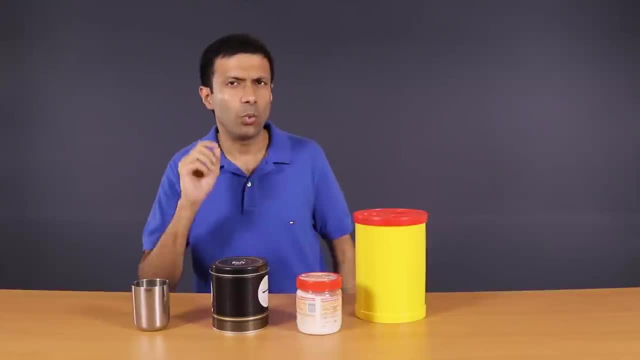 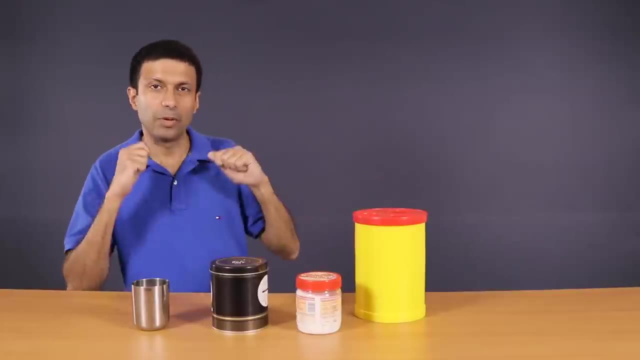 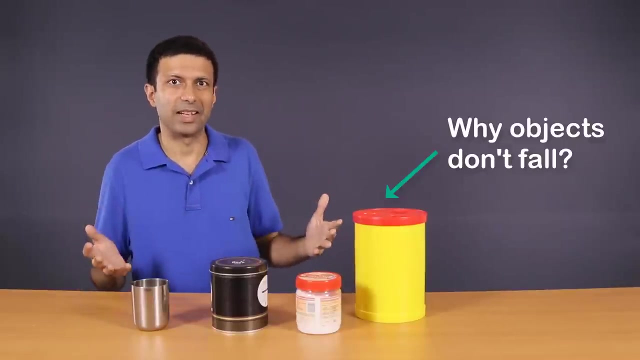 Now let's take a look at the action replay and see which Newton's law is behind this magic trick. As you saw there, when I pulled the tablecloth really quickly, these things hardly moved or didn't fall. So how do you explain that? 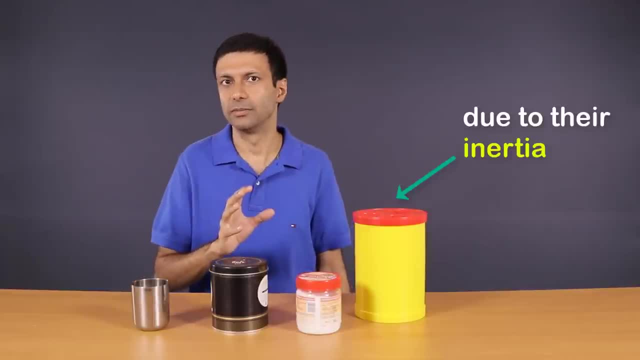 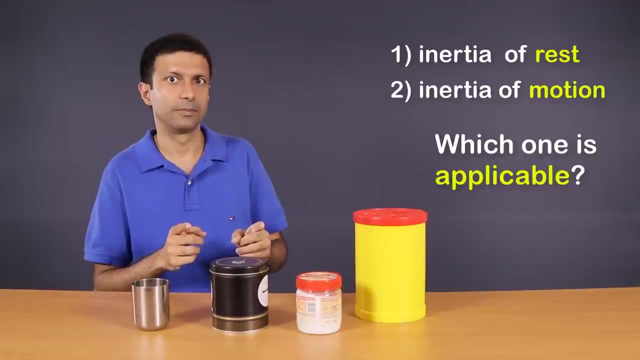 That's right, It's due to their inertia. Inertia is the laziness of a body. Now, there are two types of inertia: Inertia of rest and inertia of motion. So which one do you think is applicable in this case? That's right, It's the inertia of rest. 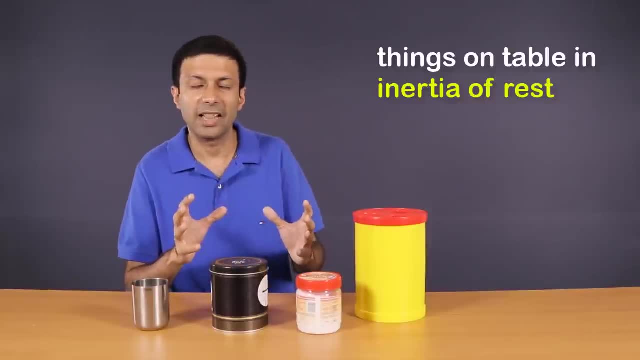 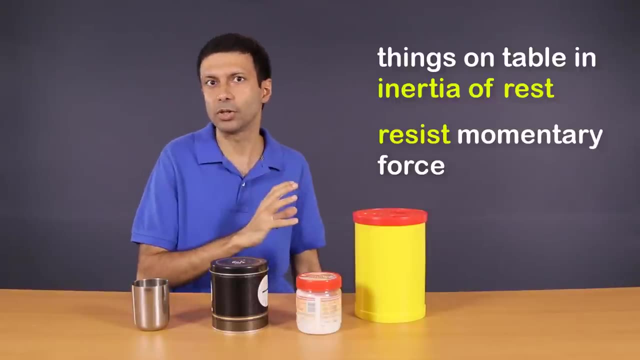 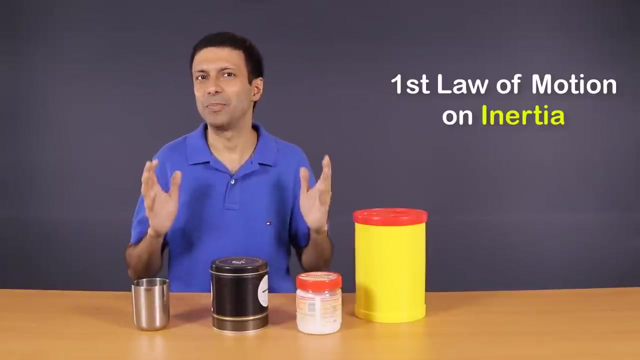 The things on the table were at rest and they want to remain at rest. So when I pull the tablecloth really quickly, they resist that momentary force and that's how they don't fall. So Newton's first law regarding inertia explains this example. 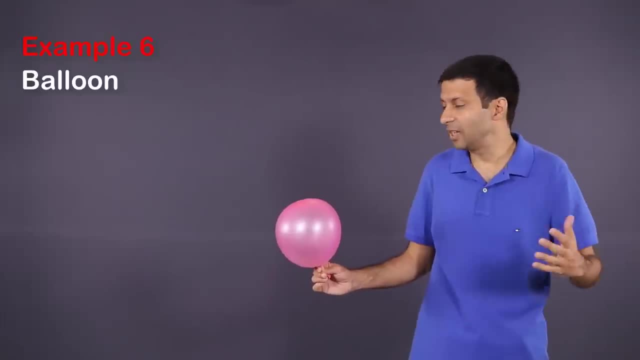 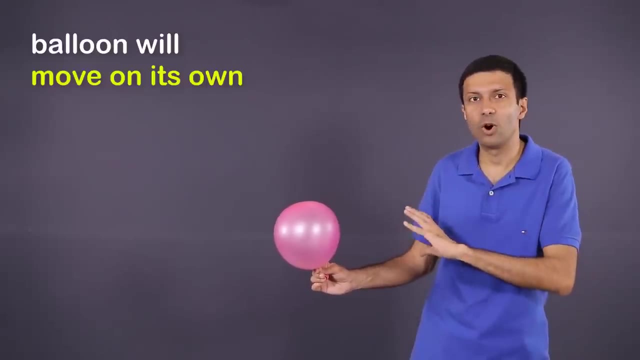 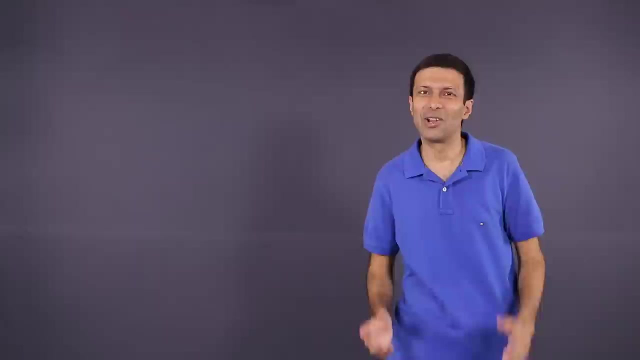 Let's see what we can learn from this balloon. here. I'm going to release this balloon and you'll see that it moves around on its own. So are you ready? Let's start Now. let's take a look at the action replay. 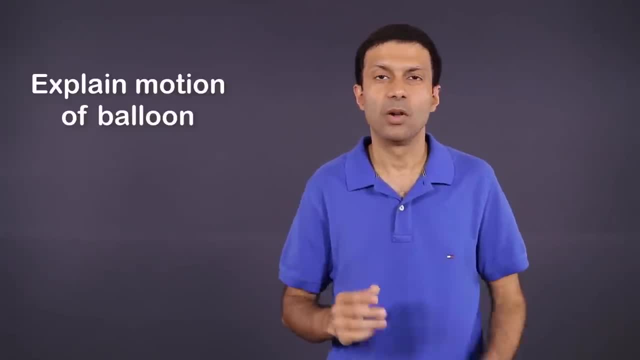 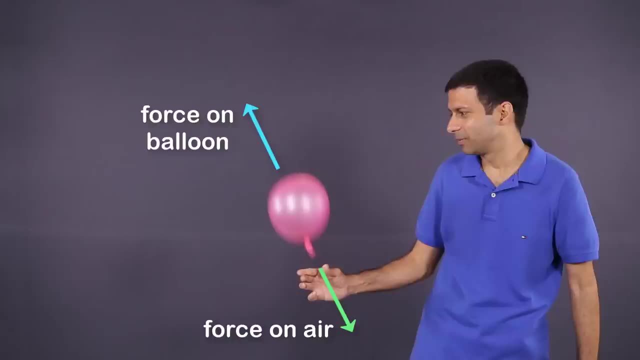 So how do you explain the motion of the balloon When I released it? the balloon pushes out the air inside. The balloon pushes out the air inside it with a force. The air exerts a force on the balloon, making it move forward. Now, are these forces equal and opposite? 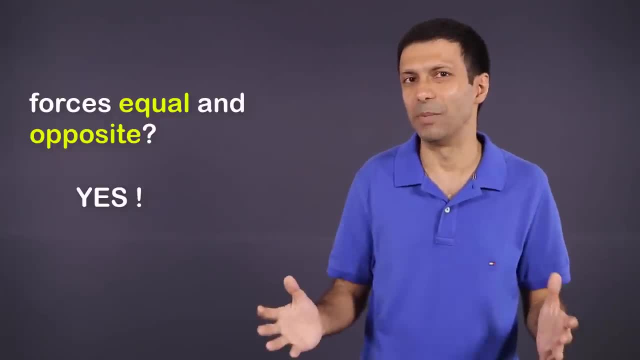 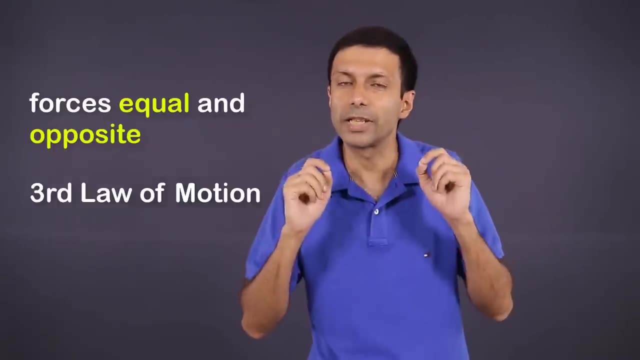 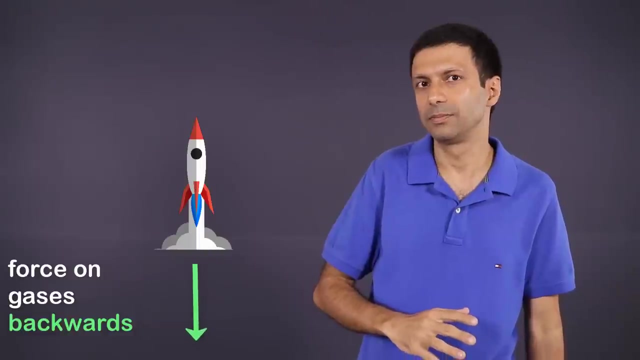 Yes. So which law are we talking about? That's right, It's Newton's third law of motion, And this same law explains how a rocket works. A rocket exerts a force on the gases backwards, And the gases exert an equal and opposite force on the rocket forwards. 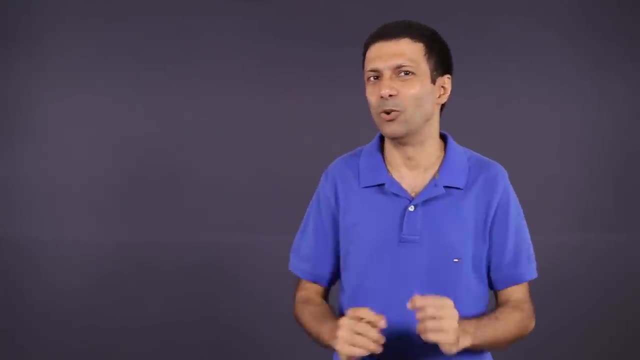 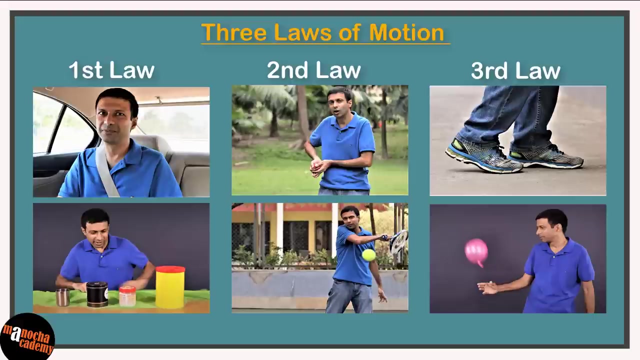 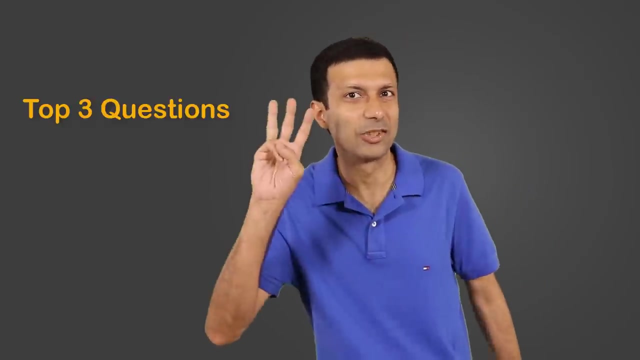 Making the rocket move, Just like this balloon. So here are the six simple, everyday examples we looked at for Newton's laws of motion. Now that we are done with the three laws of motion, are you ready to take a look at the top three questions on this topic? 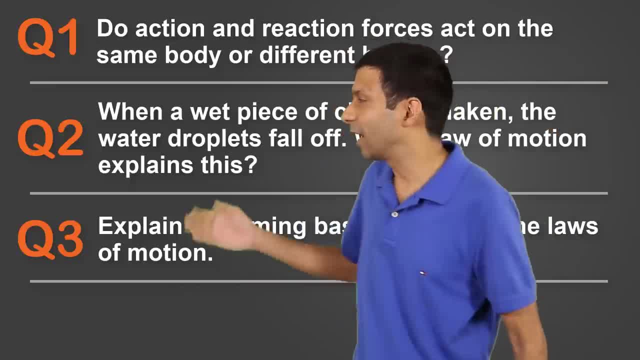 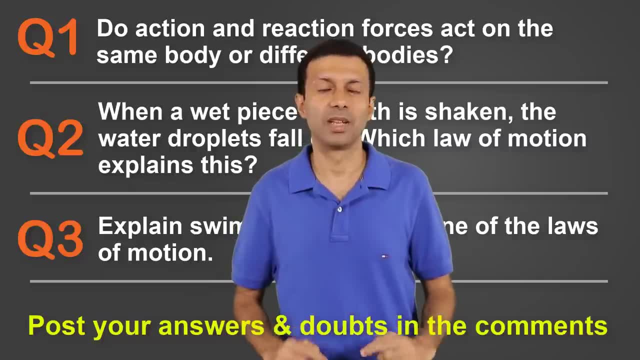 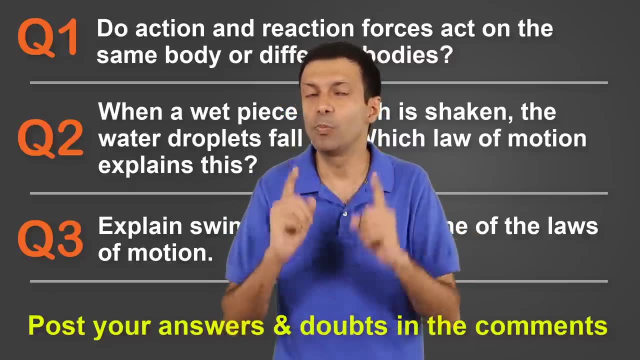 Yes, Friends, I would like you to try solving these questions And do post your answers and doubts in the comments below. I promise to reply to your comments as soon as possible, So I'll move away and you pause the video and give these questions a shot. 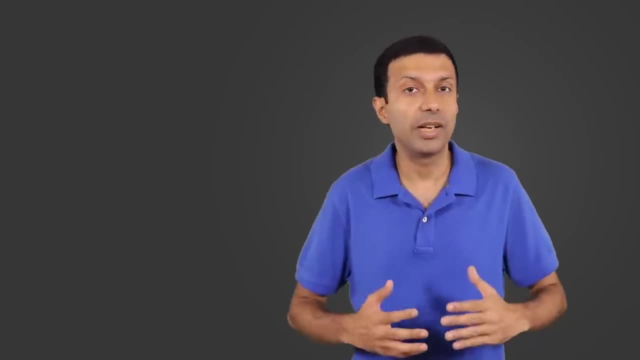 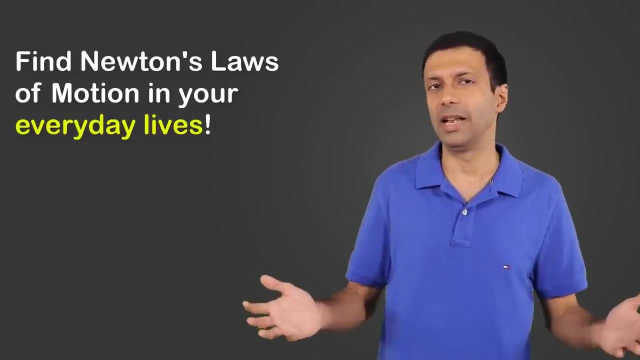 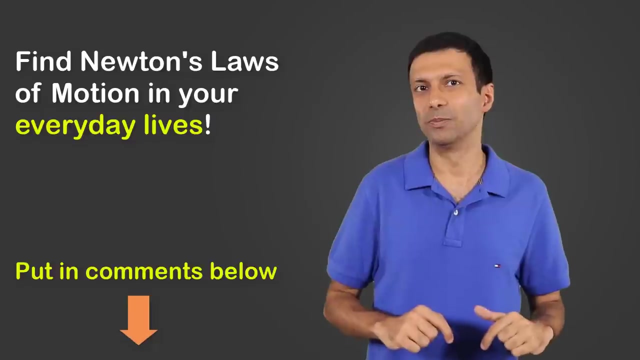 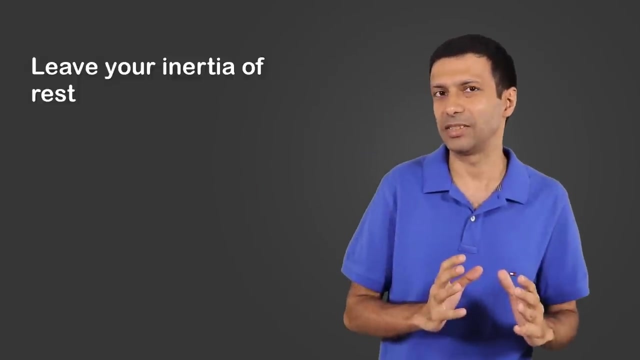 I hope you enjoyed watching the video. I would encourage you to look around and see if you can find Newton's laws of motion in your everyday lives. Do let us know what examples you experienced. by putting it in the comments below, Inspired by Sir Isaac Newton, I'm going to tell you to leave your inertia of rest. 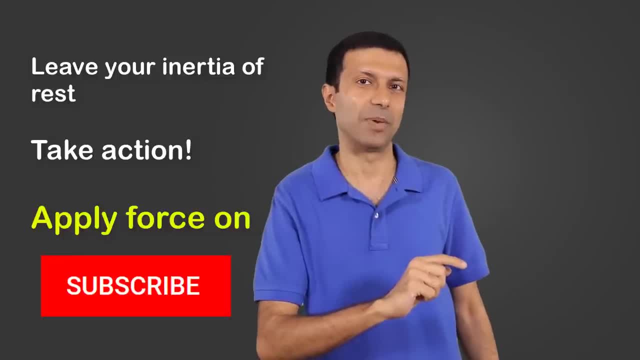 Take action and apply your force on the subscribe button, And my reaction is going to be: Thanks for subscribing to my channel.